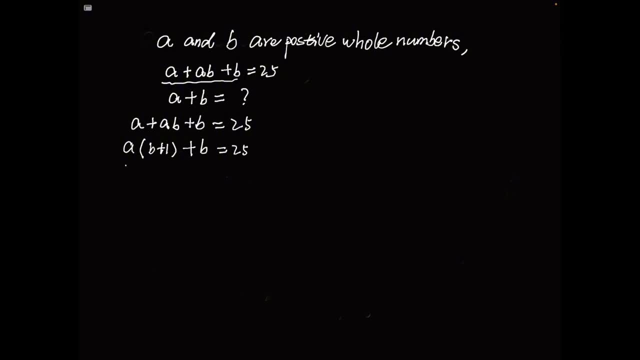 For this equation we can plus one to each side, For plus one to the left. so left side, the a, parentheses b, plus one And another. So plus one this side. So you want to keep it in balance. So we should have plus another one to the right right. 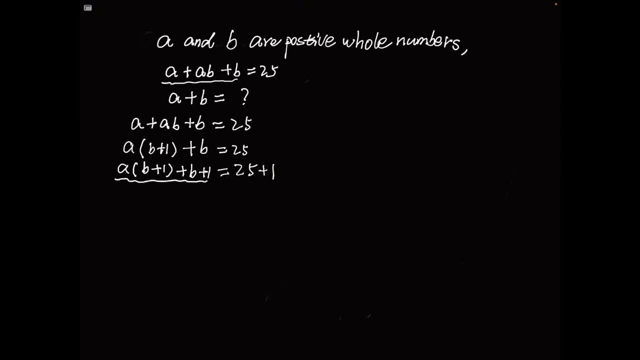 So for this left side, so we can take out the common factor. so b plus one- And outside the parentheses, is a plus one equals 26.. So this one. now we break it down, this left side impression, into the product, but two impressions. and we also know, according to the 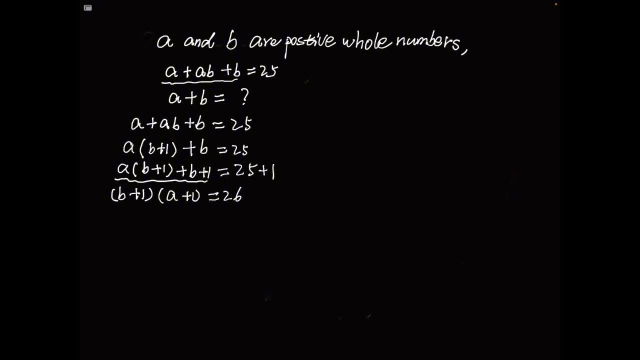 first condition: a and b are positive whole numbers. so now a plus one is greater than or equal to two, right. so b plus one. b plus one: also greater than or equal to two, right. okay, so we know we affect 26, we know 26 one it's a here. we factor at two right, so it's a 13, so so we can. 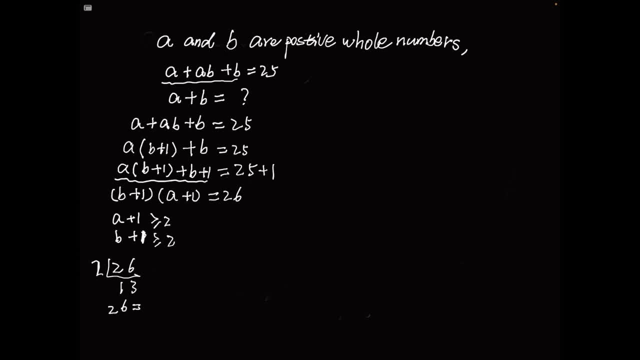 break down 26 as two numbers product, it's a 2 times 13, right? so it means one number, only one solution, right? only one solution. two numbers product. so it means one a plus one and b plus one, one, b, two. another one b is 13, right? oh, let's perform the classification and the discussion, okay, if? if b plus 1 equals 2, 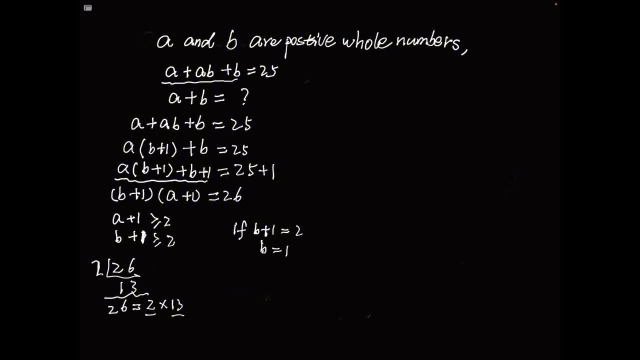 so b equals 1 and in this edition a plus 1 equals 13, so a equals 12 right. so a plus b equals 13.. the second solution: if: if b plus 1 equals 13, so b equals 12.. another terms: a plus 1 equals. 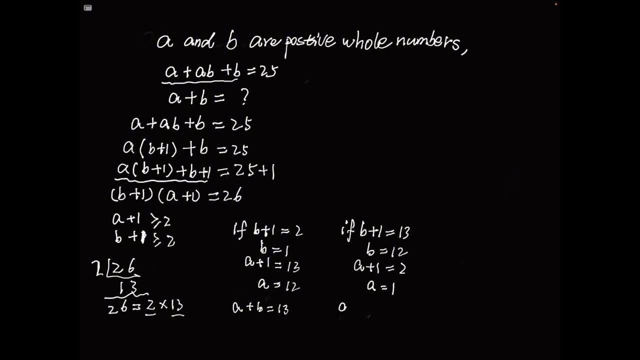 2 a equals 1 a plus b in this region equals 13. right, so now we solve. solve this question.